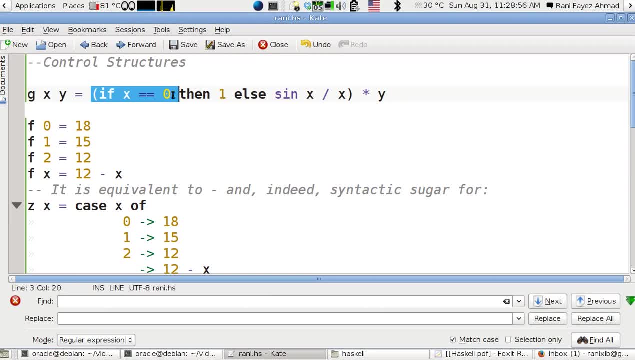 with it as a function. okay, and together here: okay. until here. this is like the result of the F statement multiplied by Y: okay, so if I input X to the function G, okay, and it was, it was zero, okay, then I should return one. why? because I can't. 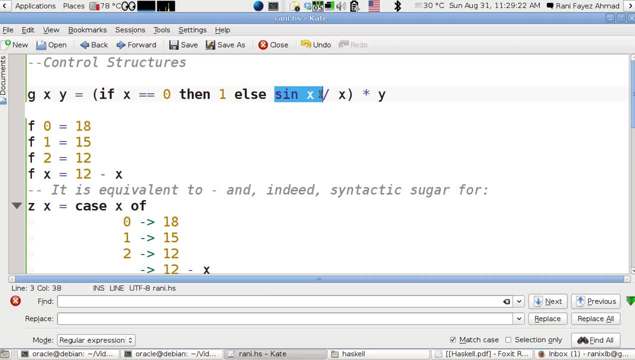 divide the trigonometric function of sine of X. okay, over X, when it's when X is zero. you can't divide by zero here, okay, so otherwise, if we input anything else other than zero, just do the division here, okay, it's a normal double floating number value, you know. so this is one of 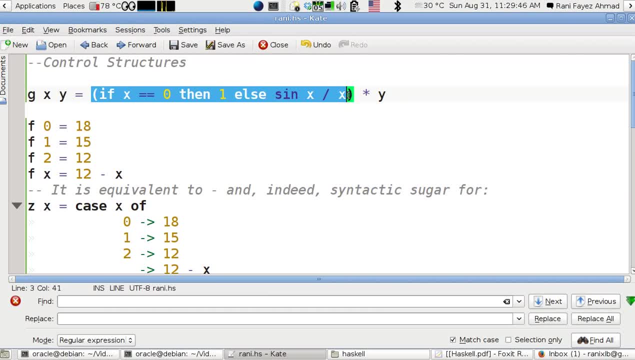 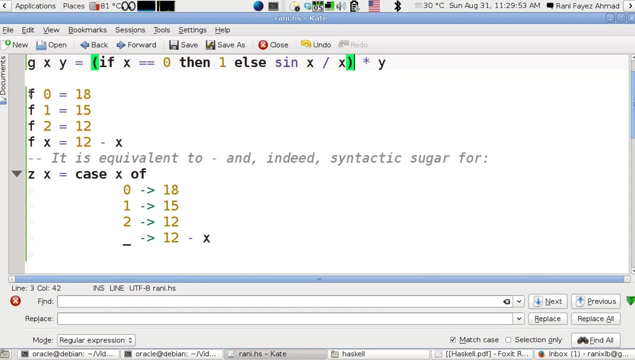 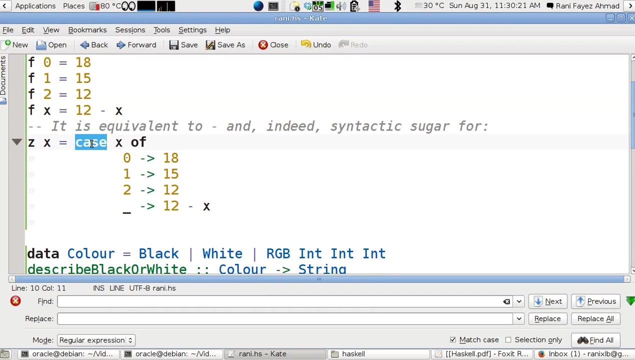 the ways to use a statement quickly. okay. now another thing is number of times. spot is equal to or equal to if I say yes. so if you do a donné something and you write that, a is a linear expression of theícula, which is very much like using the case statement of Pascal. 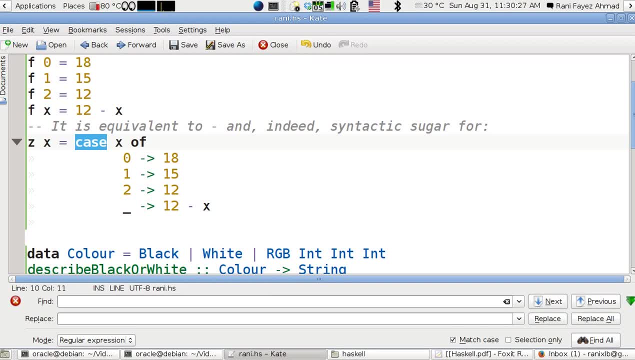 or the switch statement of Pascal, okay, of Java and C, okay. so for example, I'm saying here that for the same values on f, I just renamed it just to make it get it compiled. so z of x, okay. 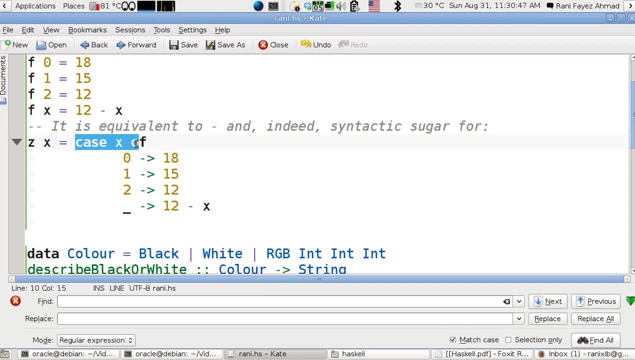 is the function of case of x of if I have 0,, I will get 18,, if I have 1,, I will get 15,, if I have 2,, it will give me 12,. so the arrow here is like: give me. 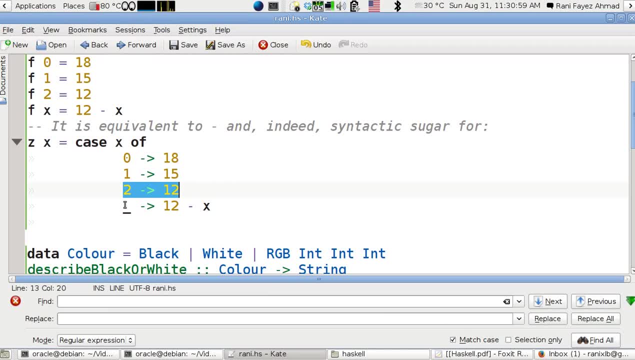 okay, it gives me the output of: okay, and you know the underscore will be whatever. okay, so by pattern matching x. if you want, you can put x here. I'm not saying you can. okay, it's like you're putting x here and 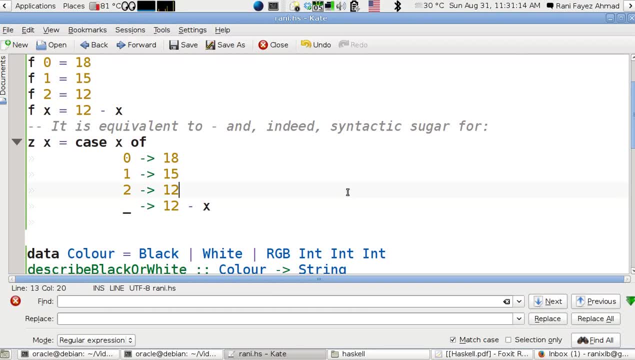 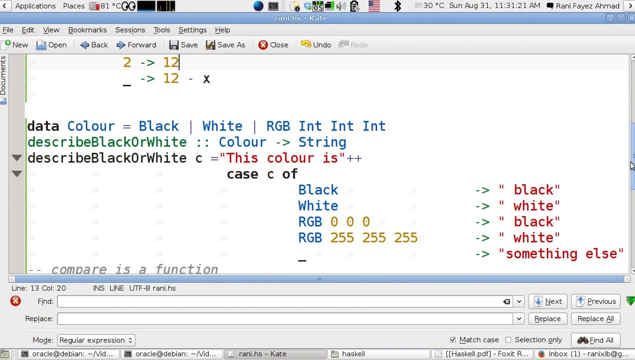 to give 12 minus x. cool, this is one way, one of the ways that you can use case. now, another way of using case is: let's imagine that I have that type called color and it gives me the constructors of a black color. 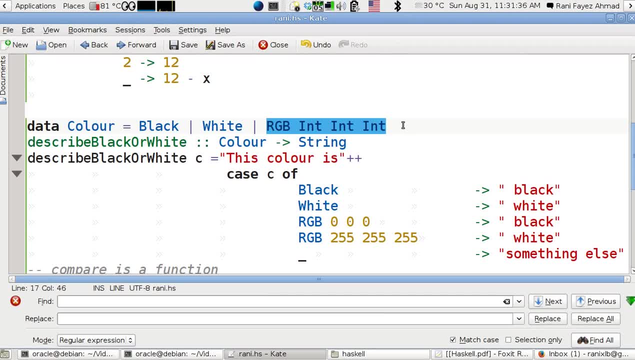 white color and any other color, using the three numbers, three integer numbers. the first integer number represents the red color. I mean, how bright is that red? okay, and how bright is that green? and how bright are then this blue? okay, the mixture of those three numbers, okay, can give you the color. 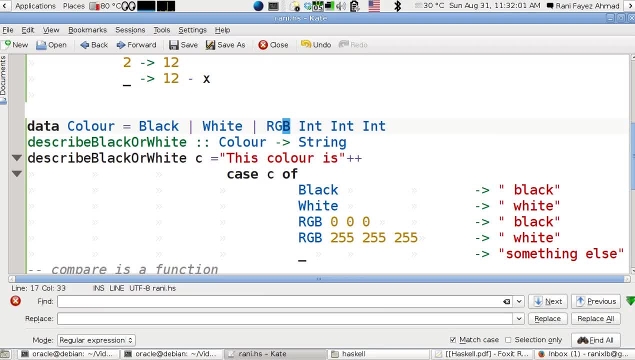 that you want. maybe you can get a velvet or violet, you know, or maybe some yellow. okay, those you can get unless you mix the R and G and B. okay. there are other ways of getting pink colors also okay, but this is one of the most. 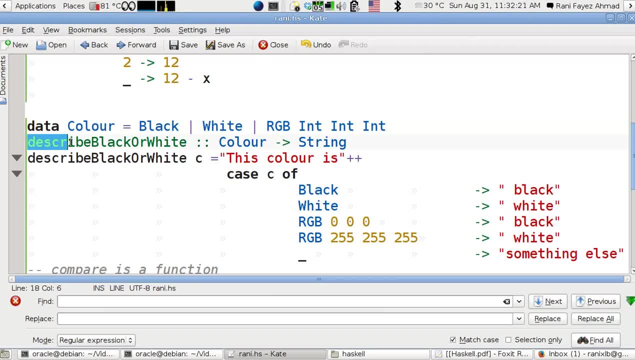 famous ones. okay, now I want to make a function that describes black or white. so it takes a color, it does not take. you know the usual. and what do you call them? native? I mean the string and integer, and you know the char. 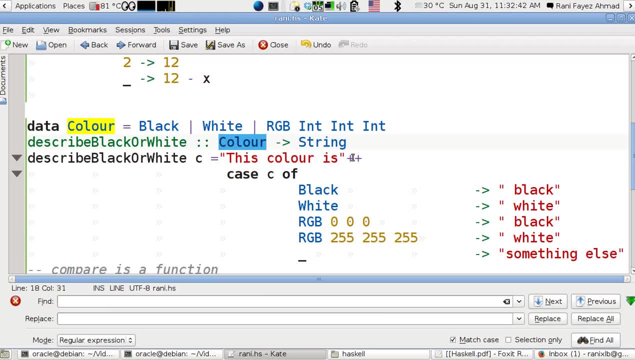 okay, so those are the primitive ones. this is the other. one say they are the primitive date types. know, here I'm putting a color. okay, so I can switch on a color. I can use a case on the color so describe black or white. 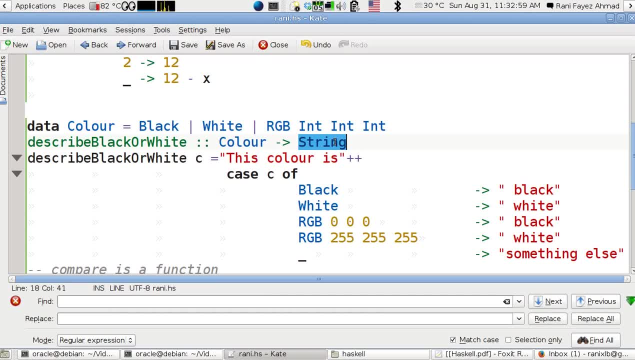 Now you know it takes a color and gives me back a string just to describe what's the type of the color that I'm input this, or whether it's a black or white. so when C is input, this color is, you're adding a string that describes the color. okay, 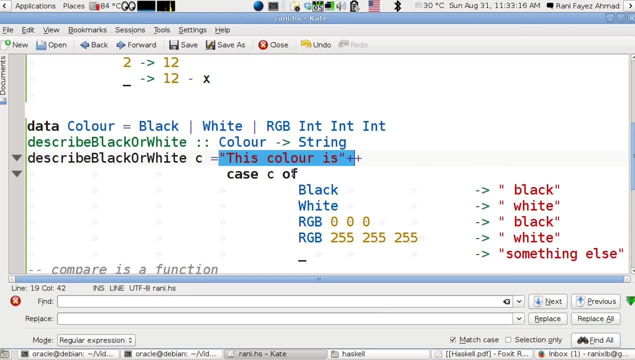 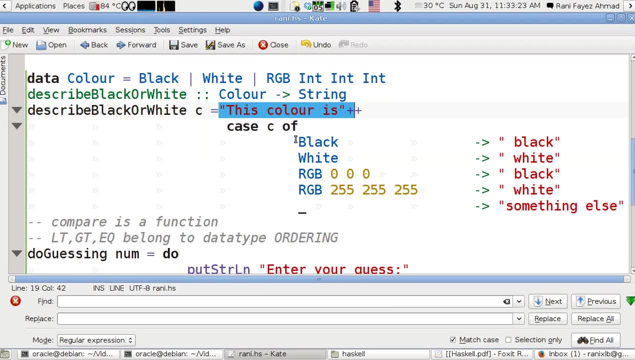 case, or see of see what's the case of c. okay, nice words, nice, uh rap. so, uh, black. it gives me a black string. okay, uh, white, gives me the word white. okay, a rgb of zeros. this is by definition. it's black. okay, you know, you made everything. 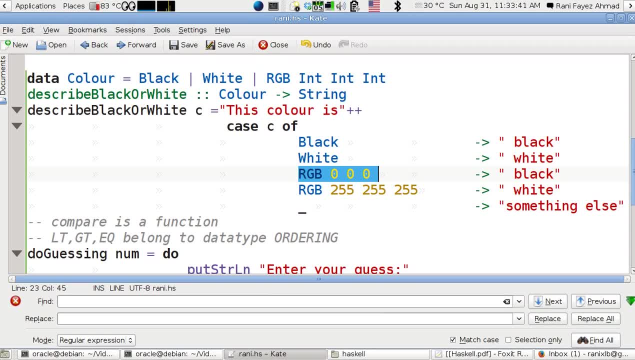 uh, dimmed, zero, okay, so it will be black. so the mixture of them, them, them, it will be zero. and the mixture of all bright, okay, 255 means the brightest ever, okay, the brightest possible, of a color. it will be white, white, white, okay, so everything will be white. 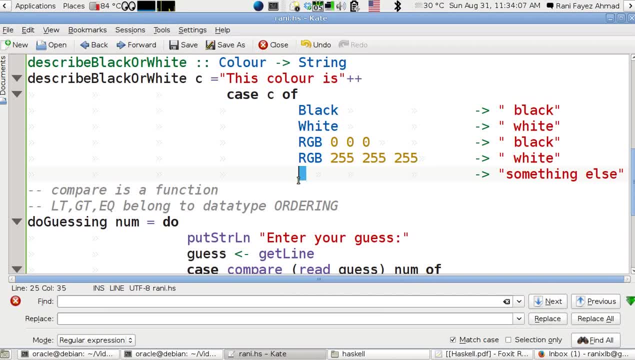 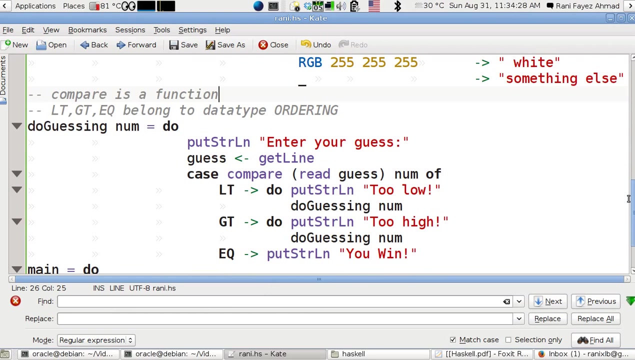 so if i use the underscore, it will be anything else. so if i have an rgb of, for example, 15, 12, 200, okay, you'll find that color, okay, so anything else will give you the word or the sentence, something else, okay. now, another way of using the case is there's a function called compare. see, i'm using it here and 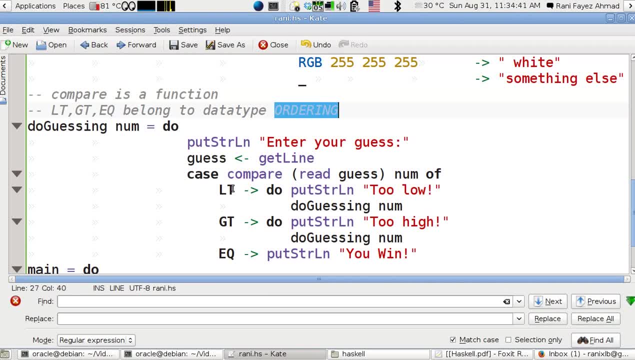 there's also a dot type called ordering. okay, and compare gives me an output of ordering okay, and the ordering can be lt for less than, gt for greater than and eq for equality. i think you guessed them. okay now, and lt and gt and eq are, you know, constructors? okay, of the ordering data type. 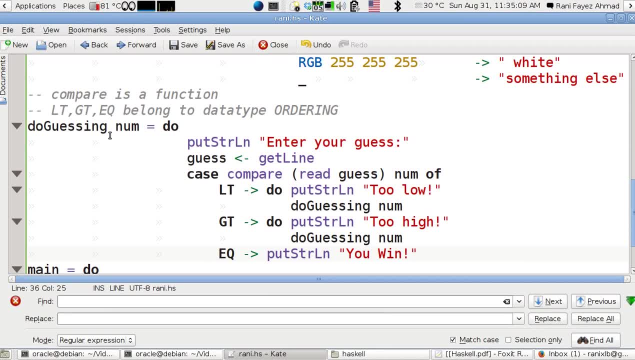 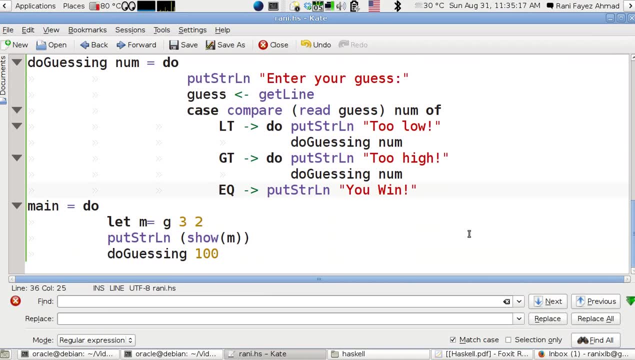 now here: what. what is he doing in this function is that he's always calling do guessing okay on the number that i've just set inside my code. like i start, for example, in the main function with do guessing as 100. now when you compile it, you give it to somebody. he doesn't know that there is. 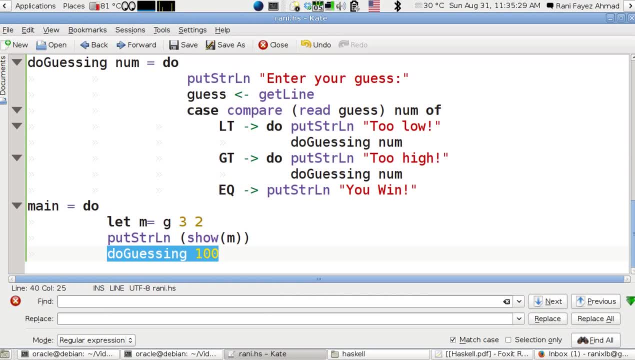 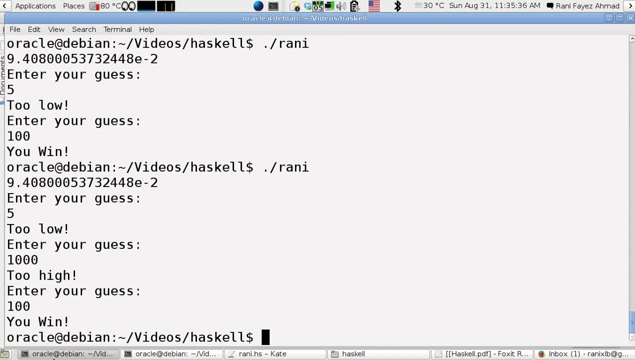 100 inside the code, so it will always call itself until you have it correctly equal to 100. okay, see, this is a test here. now, um, this is just for the uh sine over x. okay, just discovered. now. this is your interior guess. if i put one, it will be too low. it will call again the function. do guessing if i put. 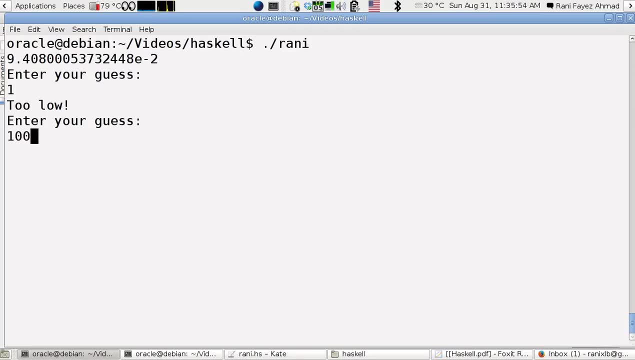 like thousand, it will be too high, okay, but 2000, it will always say to you it's too high, but i put 100, it would say you went on your group, you go out of the application, okay, all of this, so you're going to. you're going to be doing the same thing again.